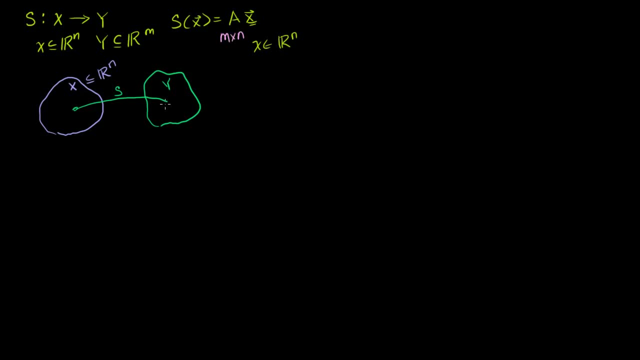 And I've told you it's a linear transformation And you'll get to some value in set y, which is in rm, And I said that the matrix representation of our linear transformation is going to be x, All right, going to be an m by n matrix, right? 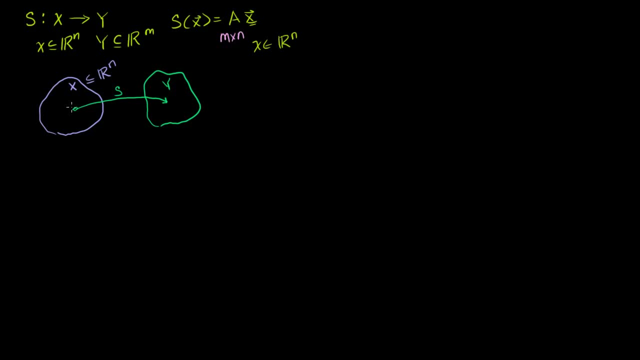 Because you're going to start with something that has n entries, or a vector that's a member of Rn, and you want to end up with a vector that's in Rm. Fair enough. Now let's say I have another linear transformation, T and. 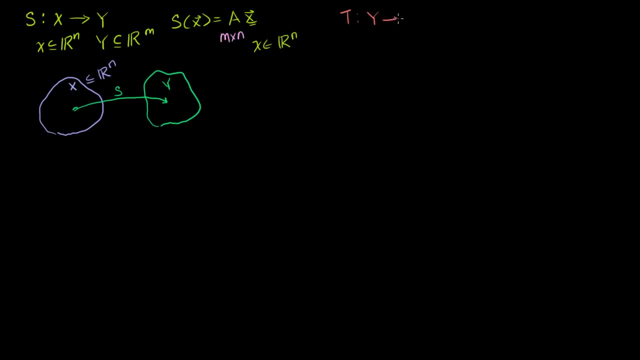 it's a mapping from the set Y to the set Z. So let me draw. So I have another set here called set Z And I can map from elements of Y. so I can map from here into elements of Z using the linear transformation T. 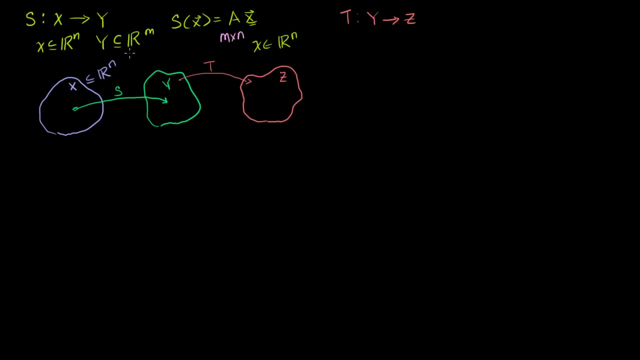 So, similar to what I did before, we know that Y is a member of Rm, We know that this is a subset, not a member more of a subset- of Rm, And these are just arbitrary letters. This could be 100 or 5 or whatever. 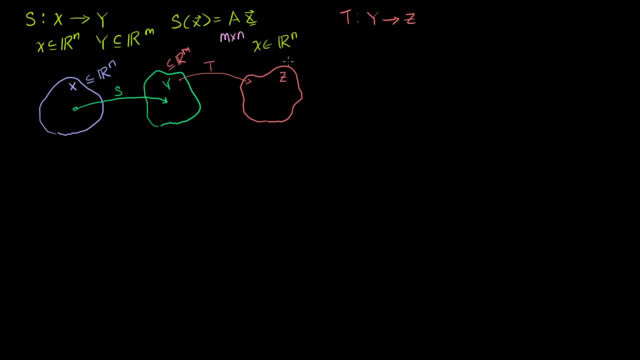 I'm just trying to stay. Let's say abstract. Now, let's say that Z is a member. I'm running out of letters. Let's say Z is a member of R, Z is a member of Rl, Then what's the transformation T, what's its matrix? 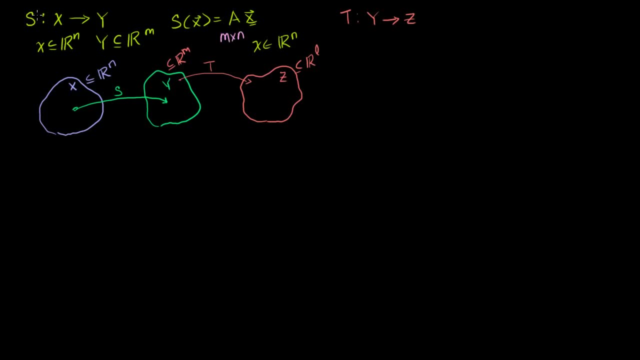 representation going to be, And we know it's a linear transformation. I told you that So we know it can be represented in this form. So we could say that T of X, where X is a member of Rm, is going to be equal to some matrix B. 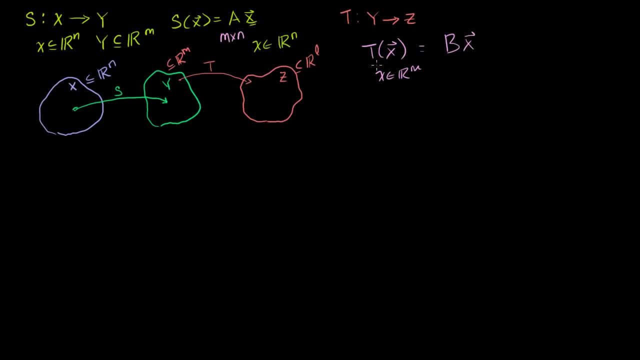 And what are the dimensions of matrix B going to be? X is going to be a member of Rm, So B is going to have to have m columns And then it's a mapping into a set that's a member of Rl. 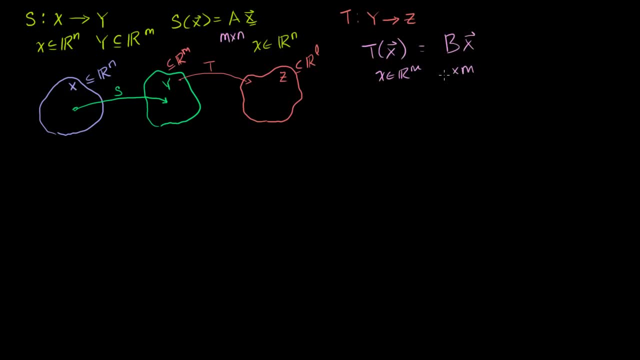 So it's going to map from members of Rm to members of Rl, So it's going to be an l by m matrix right there. Now, when you see this, a very natural question might arise in your head: Can we construct some mapping? 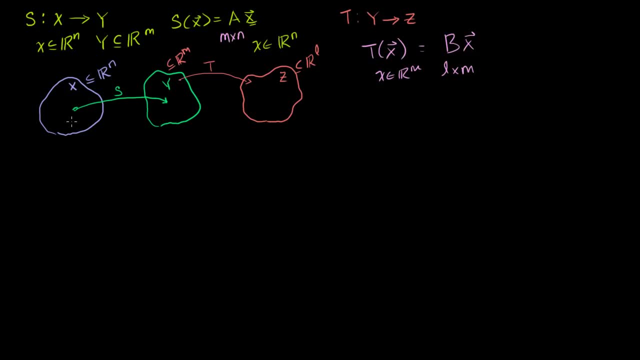 That goes all the way from set X, all the way to set T, And maybe we'll call that the composition of, and maybe we can create that mapping using a combination of S and T. So let's just make up some word. Let's just call T with this little circle S. let's just 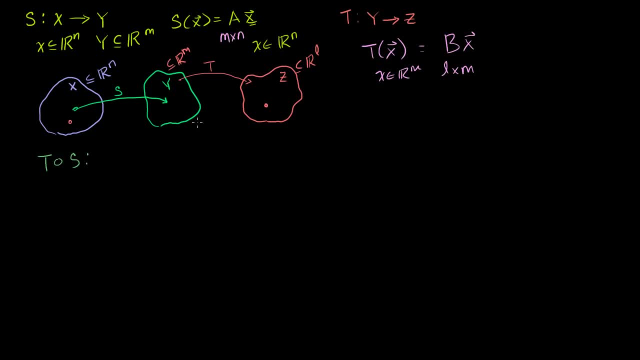 call this a mapping from X all the way to Z, From X all the way to Z, And we'll call this the composition of T with S. We're essentially just combining the two functions in order to try to create some mapping that takes us from set. 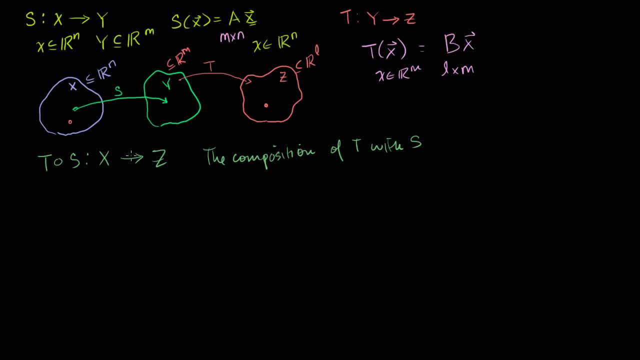 X all the way to set Z, But we still haven't defined this. How can we actually construct this? Well, a natural thing might be to first apply the set X to the transformation S. Let's say that this is our X we're dealing with right here. 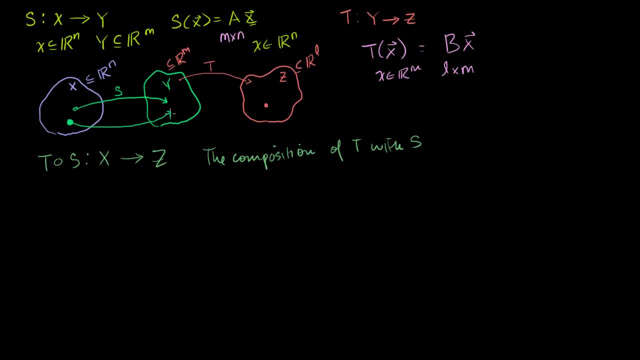 Maybe the first thing we want to do is apply S, and that'll give us an S of X, That'll give us this value right here, that's in set Y. And then what if we were to take that value and apply the transformation T to it? 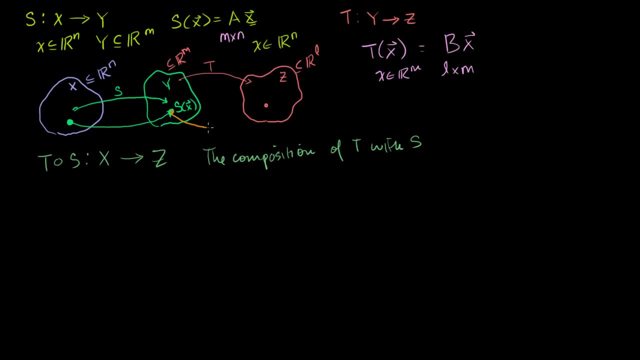 So we would take this value and apply the transformation T to it to maybe get to this value. So this would be the linear transformation T applied to this value, This member of the set Y, which is in RM. So we're just going to apply that transformation to this guy. 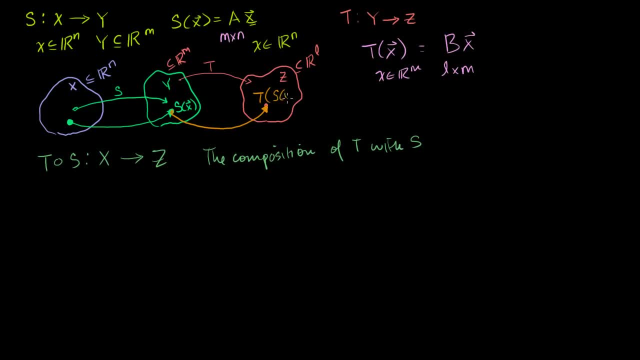 right here, which was the transformation S applied to X. This might look fancy, but all this is remember. this is just a vector right here in the set Y, which is a subset of RM. This is a vector that's in X. 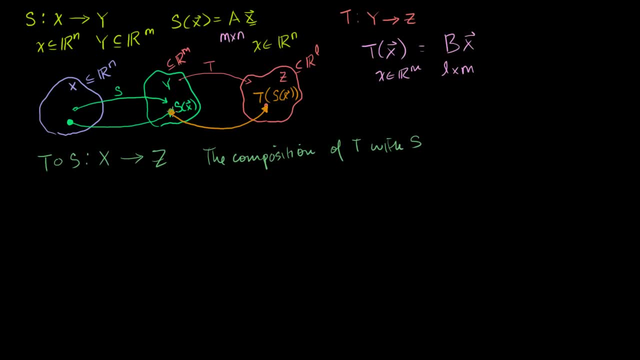 So when you apply a mapping, you get another vector that's in Y and then you apply the linear transformation T to that, And then you get another vector that's in set Z. So let's define the composition of T with S. This is going to be a definition. 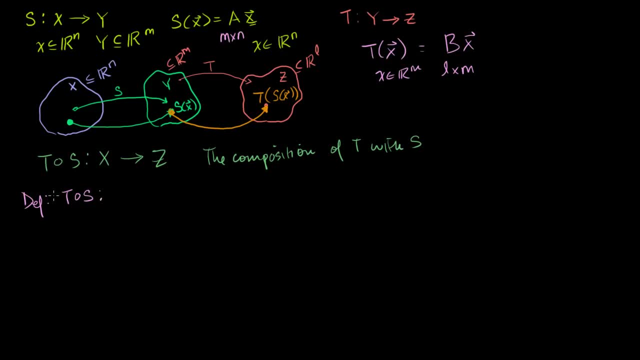 Let's define the composition of T with S to be: first we apply S to some vector in X to get us here, And then we apply T to that vector to get us to set Z. So we apply T to this thing, right there. 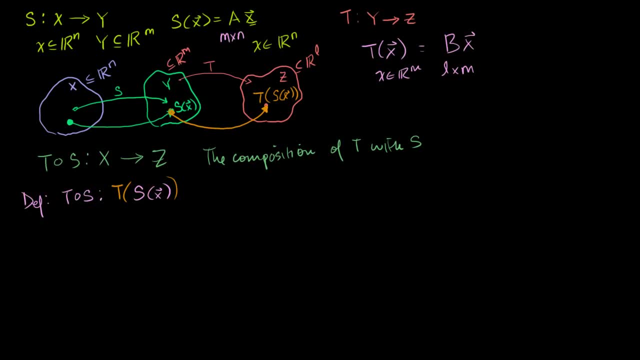 Now the first question might be: is this even a linear transformation? Is the composition of two linear transformations even a linear transformation? Well, there are two requirements to be a linear transformation right: The sum of the linear transformation, of the sum of. 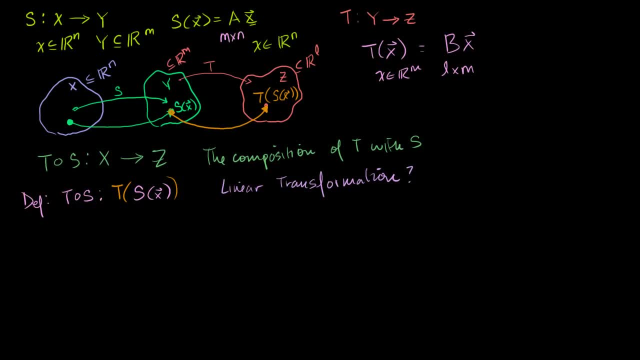 two vectors should be the linear transformation of each of them summed together. So let's see What I know. when I just say that Verbally, it probably doesn't make a lot of sense. So let's just try to take the composition of T with S of. 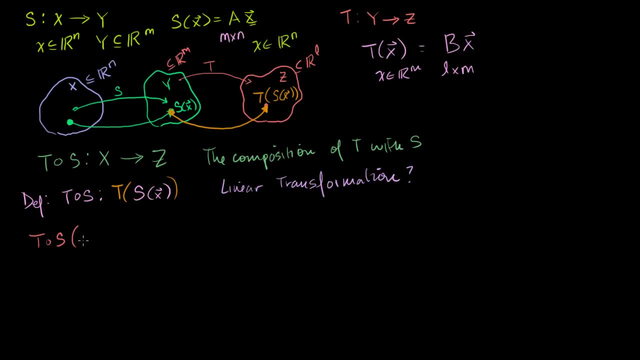 let's say the sum of two vectors in X. So let's say I'm taking the vectors X and the vectors Y. Well, by definition, what is this equal to? This is equal to applying the linear transformation T to the linear transformation S applied to our two vectors X. 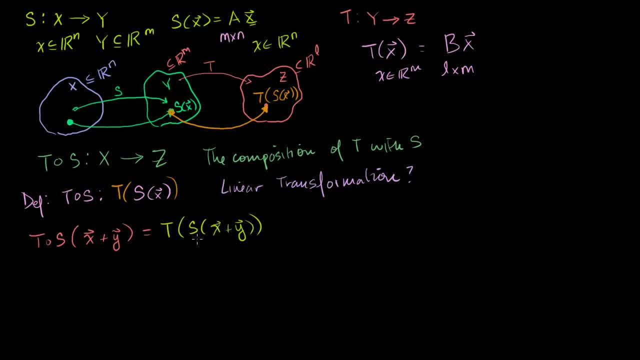 plus Z, And what is this equal to? I told you at the beginning of the video that S is a linear transformation. So, by definition of a linear transformation, one of our requirements- we know that S of X plus Y is the same thing. 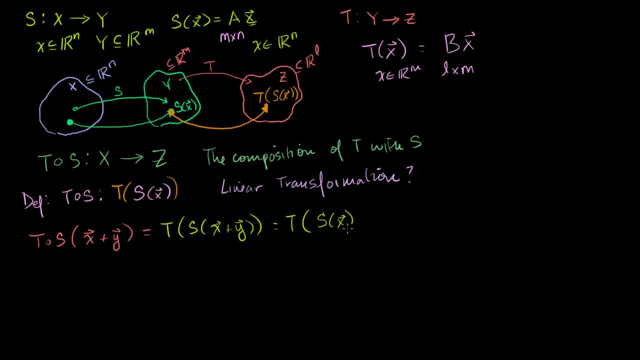 as S of X plus S of Y, Because S is a linear transformation. We know that that is true. We know that we can replace this thing right there with that thing right there. Well, we also know that T is the linear transformation which. 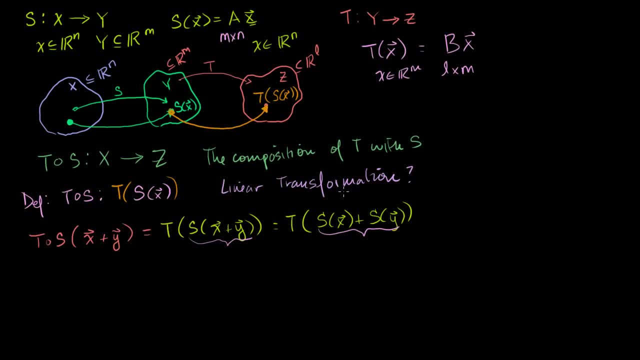 means that the transformation applied to the sum of two vectors is equal to the transformation of each of the vectors. summed up So, the transformation of S of X Or the transformation applied to the transformation of S applied to X. I know the terminology is getting confused. 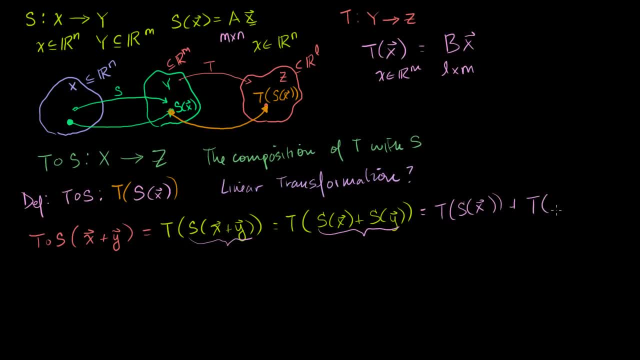 Plus T, of S, of Y. Now, what are the problems that we don't know exactly about? T? Well, there are multiple questions we don't know about. we don't know exactly why that is, But we can act: create curved toolbox. What is it? so we have to add constraints. 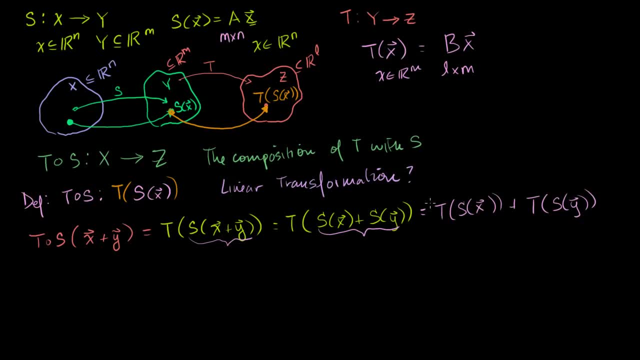 We have to specify details from the official послеoks on what is This is. we can do this because we know that t is a linear transformation. But what is this right here? This is equal to this statement. right here is equal to the composition of t with s applied to x plus the. 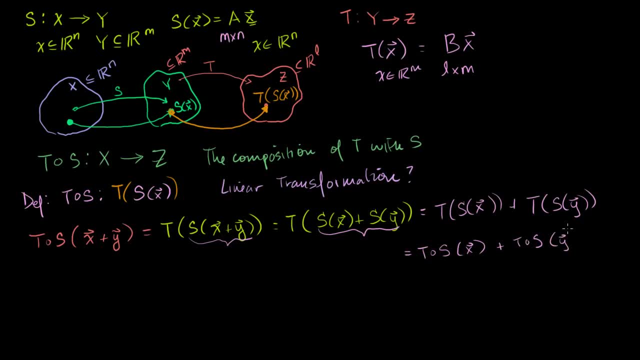 composition of t with s applied to y. So, given that both t and s are linear transformations, we got our first requirement: that the composition applied to the sum of two vectors is equal to the composition applied to each of the vectors summed up. So that was our first requirement for a linear 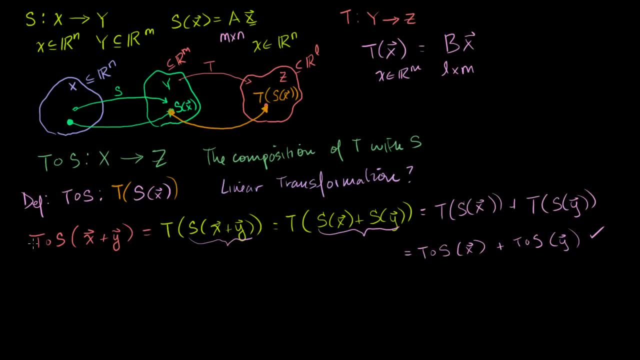 transformation. And then our second one is: we need to apply this to a scalar multiple of a vector in x. So t of s, or let me say it this way: the composition of t with s applied to some scalar multiple of some vector x. 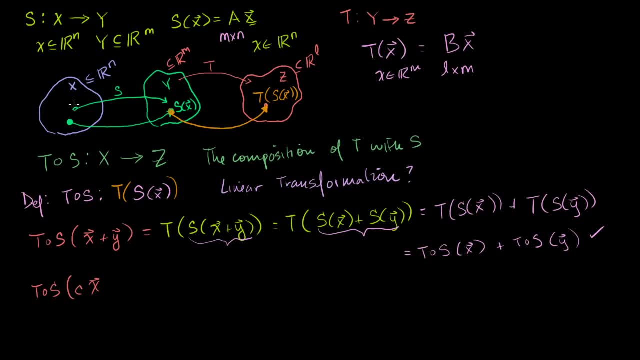 that's in our set x. This is a vector x. that's our set x. This should be a capital X. This is equal to what? Well, by our definition of our linear, of our composition, this is equal to the transformation t applied to. 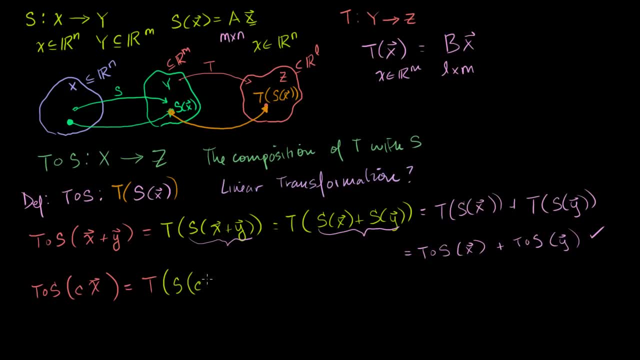 the transformation s applied to c times our vector x, And what is this equal to? We know that this is a linear transformation. So, given that this is a linear transformation, that s is a linear transformation. we know that this can be rewritten as: 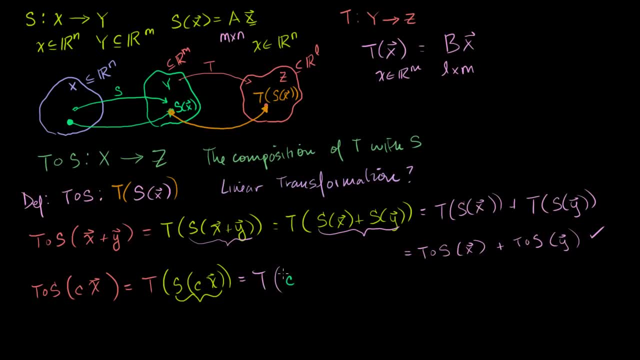 t times c. This is equal to c times s applied to x. This little replacing that I did with s applied to c times x is the same thing as c times the linear transformation applied to x. This just comes out of the fact that s is a linear. 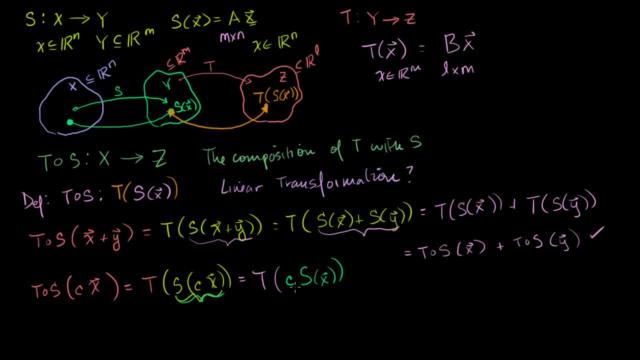 transformation. We've done that multiple times. Well, now we have t applied to some scalar multiple of some vector, And so we can do the same thing. We know that t is a linear transformation, So we know that this is equal to- I'll do it down here this: 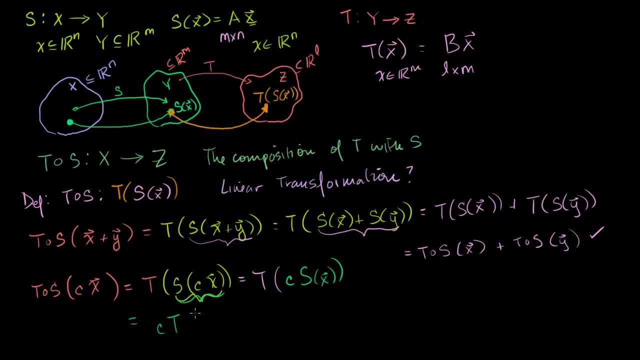 is equal to c times s. This is equal to c times t applied to s, applied to some vector x. that's in there. And what is this equal to? This is equal to the constant c times the composition t with s of our vector x, right there.